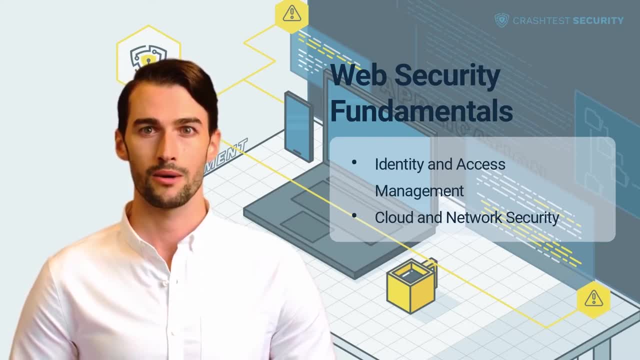 adopt the right systems to prevent cyber attacks. This article discusses web security basics, common vulnerabilities and resources to keep abreast with the changing threat landscape. security strategy to ensure all related components of web applications are secure. because of the extensive attack surface, modern tech frameworks offer security risks differ. 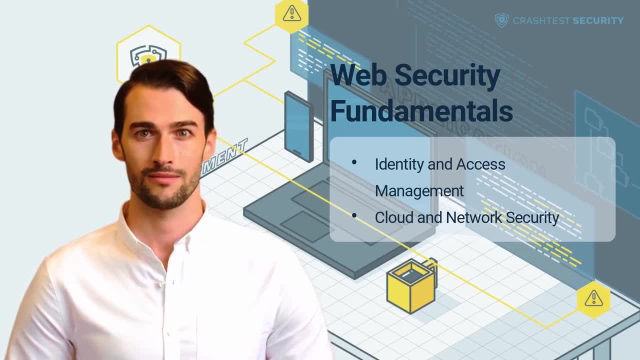 based on industry types and technologies used, however, the approach of mitigating attacks is the most common. some of these include identity and access management. identity and access management- iam- is one of the most crucial parts of web security. it forms the first layer of defense by governing permissions and access to. 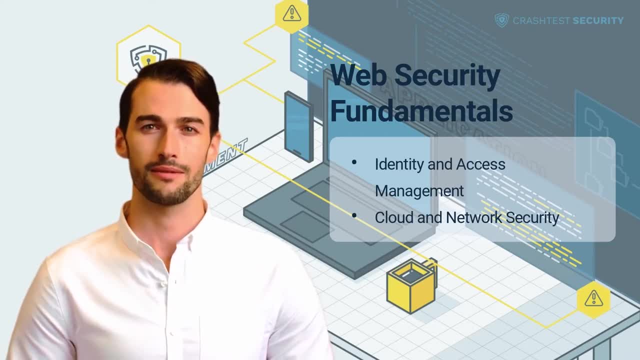 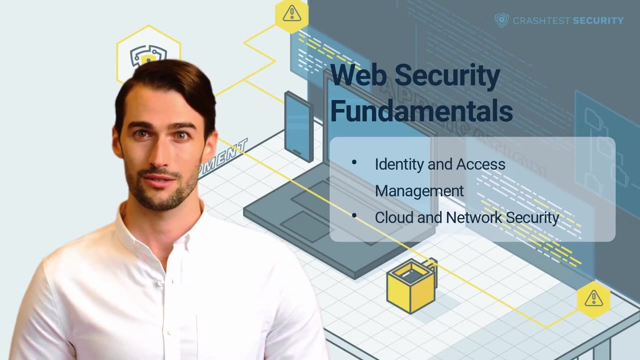 applications, data and other resources. iam involves identifying, authenticating and authorizing web application users to ensure seamless yet robustly secure access management. since iam solutions automate and streamline the core processes of access management, development teams can focus on enhancing the application's operational efficiencies, resilience and scalability. a typical iam platform also automates access reviews, log collection and reporting. 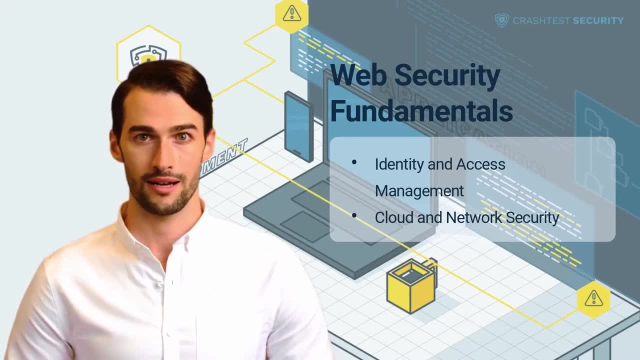 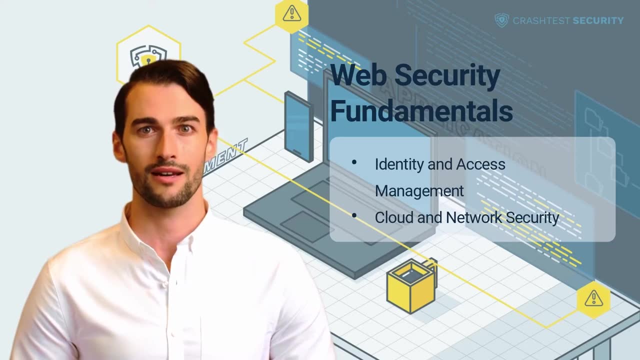 supporting regulatory frameworks and security strategies to ensure seamless and secure access to web applications frameworks compliance, cloud and network security. because of the continuous cloud adoption for hosting modern web applications, software-defined networks have witnessed unprecedented growth. most attackers utilize these networks as entry points, using a combination of tactics to compromise the information flow across the web ecosystem. 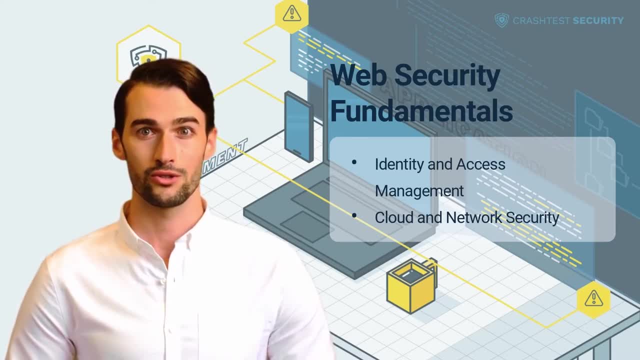 unsurprisingly, a massive part of web security now involves ensuring that data shared between distributed networks is kept secure. though cloud service providers offer inbuilt security measures through their platforms, cloud security is primarily a shared responsibility between the service provider and the end user for systems that run on hybrid public and private cloud. 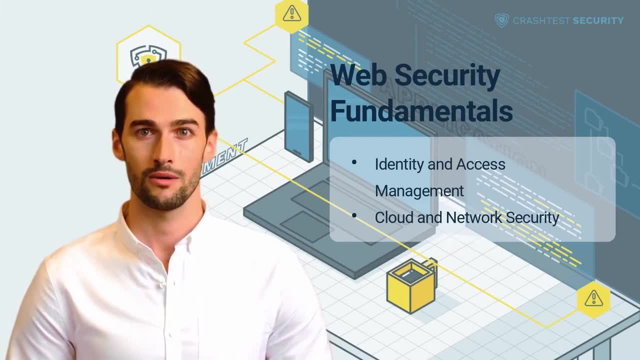 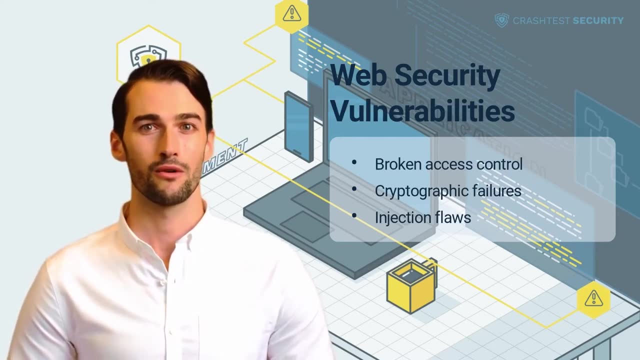 or multi-cloud architecture. provisions for developing a comprehensive security mechanism often require a complex custom approach. vulnerabilities are weaknesses or flaws that hackers exploit to compromise a system. the online web applications security project, owasp, outlines the top 10 web security measures for cloud security in the world of cloud security. 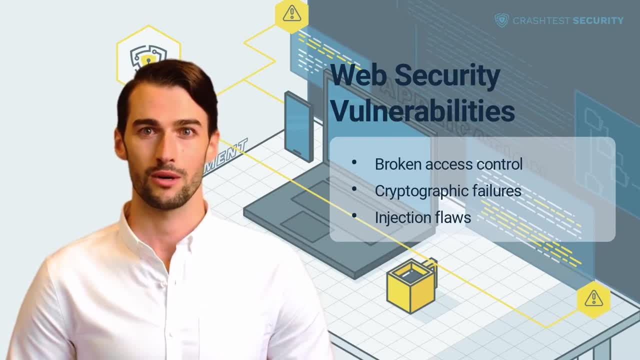 vulnerabilities in 2021 and ranks them according to exploitability, detectability and potential damage. some of these vulnerabilities include broken access control. one of the most prevalent forms of vulnerability allows users to perform actions outside their intended permissions. hackers commonly exploit various vulnerabilities of broken access control, including violating the 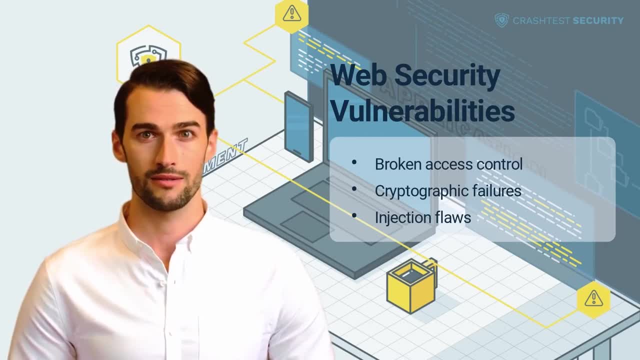 least. privilege principle, insecure direct object reference and missing controls for http methods. cryptographic failures: cryptography uses mathematical techniques to allow only the sender and intended recipient to view data. some cryptographic flaws include: transmitting data as clear text, use of weak, outdated cryptographic algorithms, use of default keys and short. 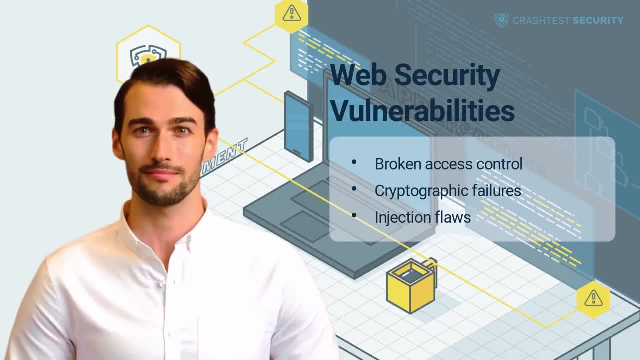 initialization vectors. injection flaws. these vulnerabilities allow attackers to use malicious scripts to infect a web server through user input interfaces. such vulnerabilities typically arise due to insufficient input validation, hostile data within the object relational model or when dynamic queries are used directly in the web server's interpreter. other owasp web application. 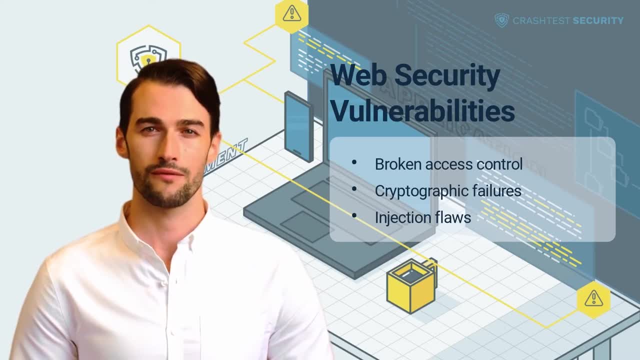 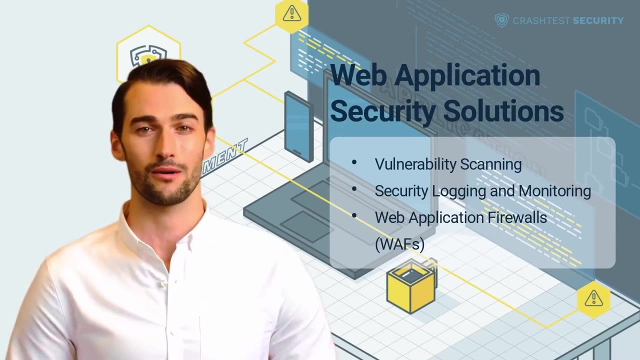 vulnerabilities include insecure design, security misconfiguration, outdated vulnerable components, authentication failures, server-side request forgery and security logging and monitoring failures. ensuring web application security is multi-faceted and spans multiple workflows, regulatory framework and knowledge areas. web security solutions integrate various services to offer customizable protection for sensitive workloads, while use cases may differ for different organizations. 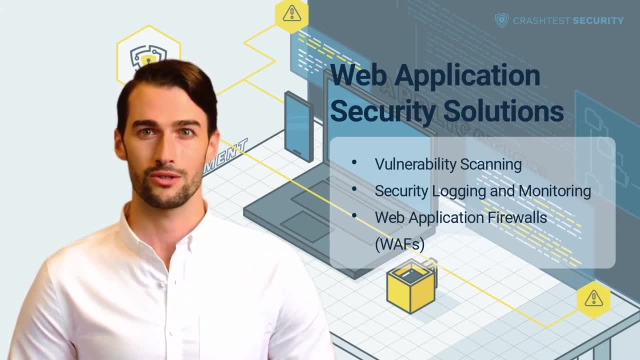 the following are some of the most commonly leveraged application security solutions: vulnerability scanning. a vulnerability scanner is a vulnerability assessment solution that automatically tests the web server's configuration, code and dependencies for security gaps. instead of being a one-time project, vulnerability scanning is a continuous process that enables distributed teams to achieve agility. 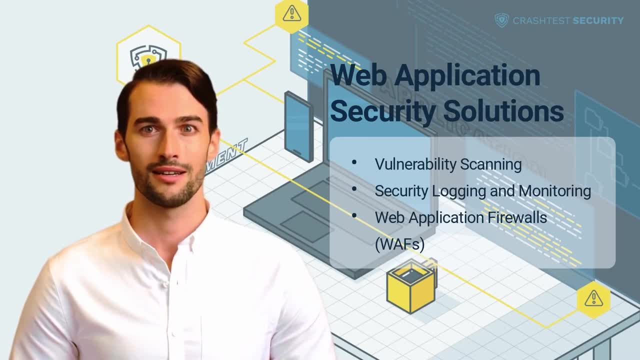 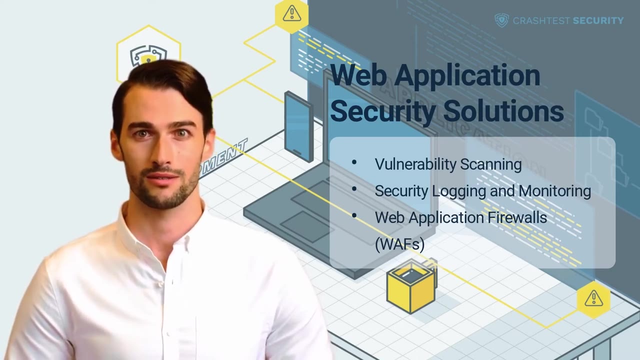 by eliminating security testing bottlenecks. besides identifying weaknesses in a tech stack, vulnerability scanning also helps security teams evaluate the effectiveness of their cyber security strategy. crash test security offers a vulnerability scanner to help eliminate security blind spots for various web applications. app is in javascript. the platform establishes an. 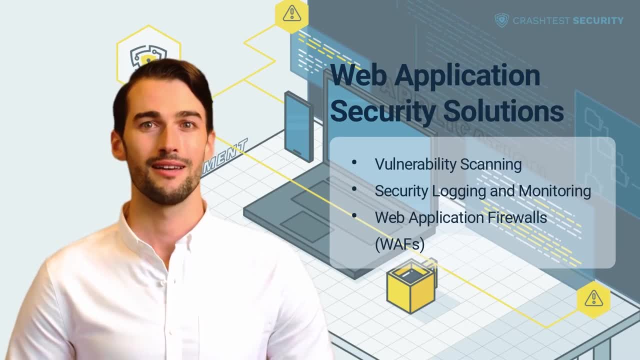 end-to-end continuous testing process by automating scanning and by enabling the support of a team of, while delivering negligible false positives and actionable reports. Sign up for a free two-week trial to see how Crash Test Security can help you with faster security assessments, Security Logging and Monitoring. 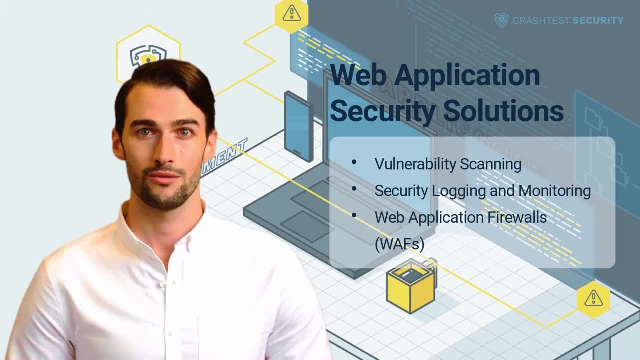 All network devices generate several events and actions recorded as logs. Log management is the process of categorizing, aggregating and assessing for evidence of abnormalities. Therefore, when implementing a cybersecurity strategy, organizations should ensure that all components of the computing network our logging events and that the logs are managed centrally to identify a root cause efficiently. 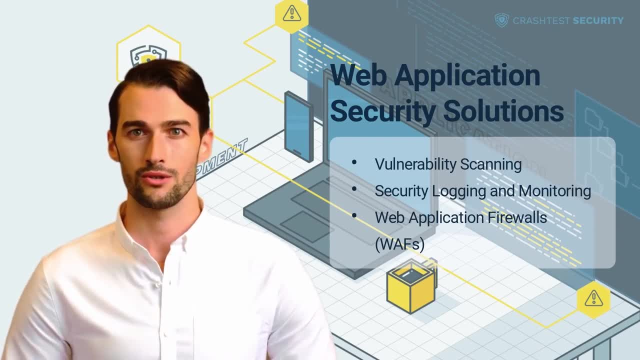 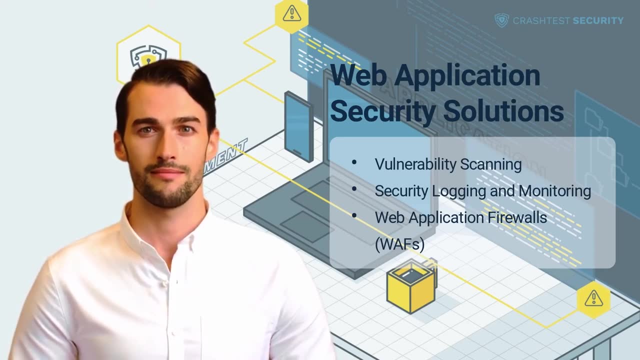 Monitoring involves using telemetry data to detect and diagnose security threats proactively. Proper monitoring tools scan the content delivery network, web servers and endpoints in real-time, enabling teams to mitigate attack vectors before hackers exploit them. Web Application Firewalls, WAFs. 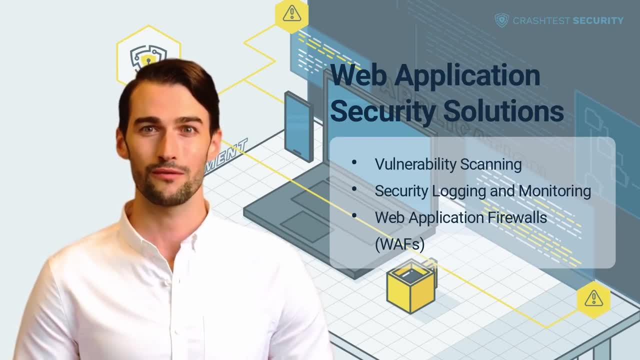 A web application firewall is a commonly used tool for protecting web applications from attacks. A WAF creates a protective shield of Layer 7 protection for a web server by applying several rules to HTTP transactions. While doing so, WAF relies on a set of policies to essentially create a blacklist or whitelist. 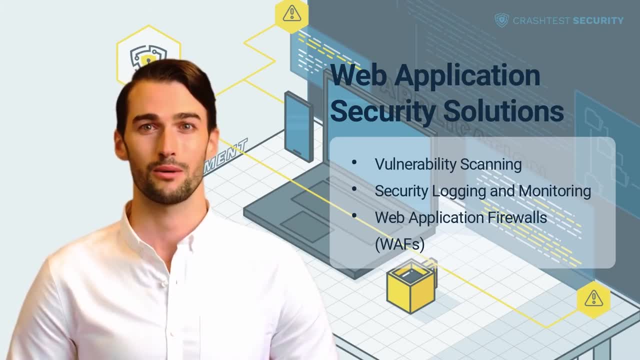 that filters out malicious code or requests from interacting with a web server. Though WAFs are primarily used to detect and block malicious requests such as SQL injection or cross-site scripting, they can also help prevent the abuse of APIs by blocking API calls that do not conform to their 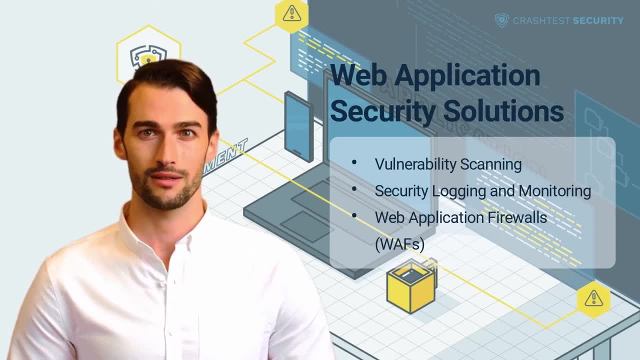 policies. A WAF can be either network-based, host-based or cloud-based. Cloud-based WAFs offer turnkey installation and are more accessible and affordable to implement. These WAFs can protect applications on-premises in the private cloud. 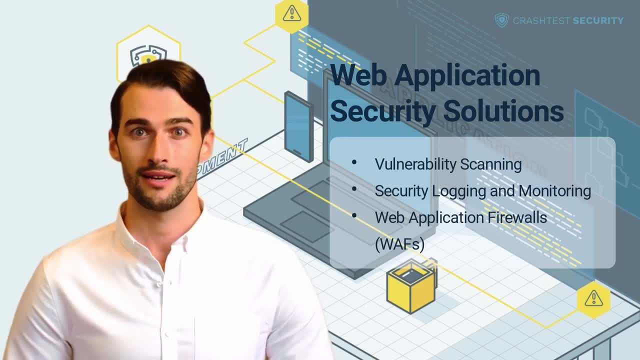 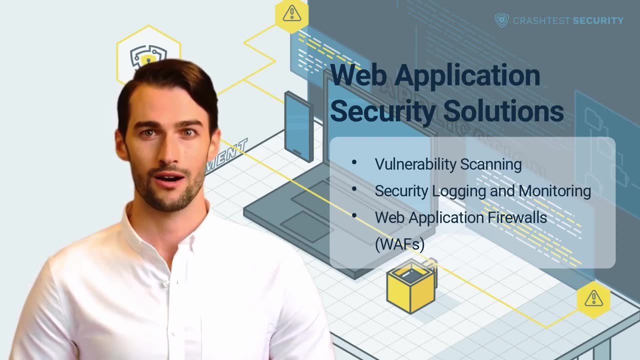 or in public offerings such as Google Cloud, Ms Azure and AWS. For example, Prisma Cloud CloudFlare and Google Cloud Armor are popular cloud-based web firewall security solutions that improve protection by monitoring and filtering traffic between the web server and the internet. 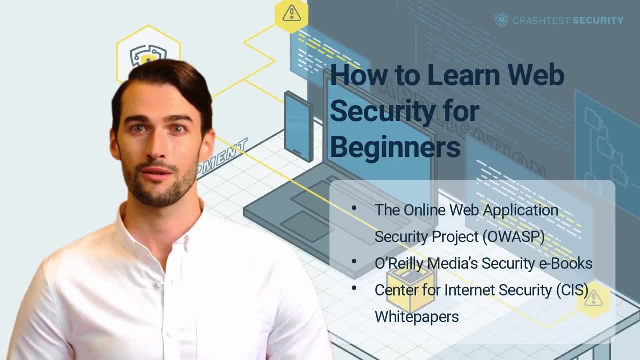 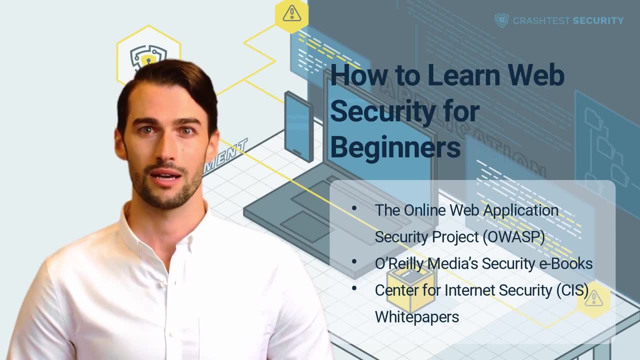 While cybersecurity is a complex and broad subject, there are numerous resources to help anyone learn web security. These include: 1. The Online Web Application Security Project. OWASP is a non-profit foundation that helps improve software security through open-source projects, conferences and community contributions. 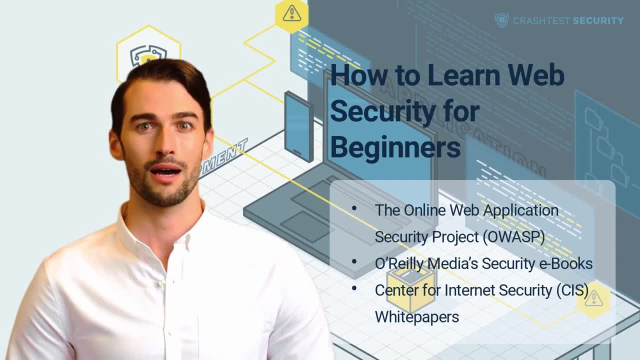 OWASP offers training, tools and resources through its vibrant community and volunteer networks. Whether you are a developer, security professional or startup founder, OWASP resources are meant for everyone looking to secure their tech stack. OWASP has various niche projects on application security, including. 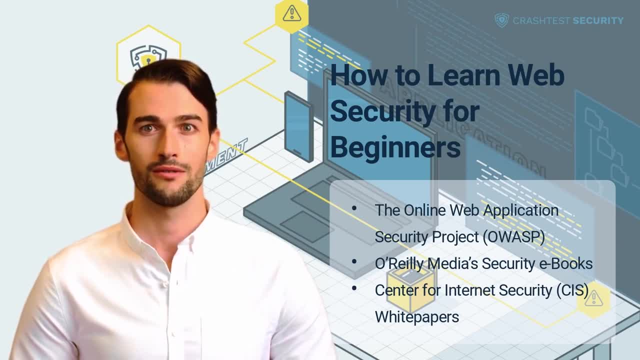 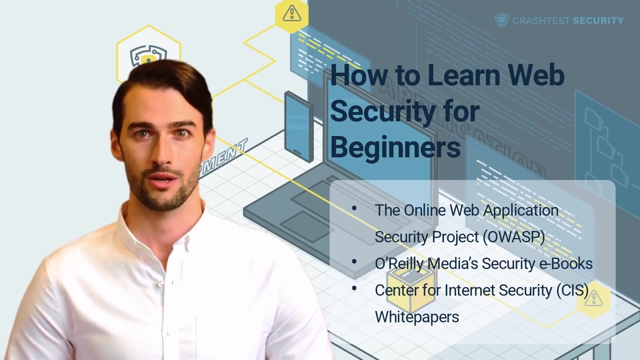 OWASP Top 10: A numbered list of common threats to look out for, along with the best practices to avoid related vulnerabilities. Web Security Testing Guide- STG- A reference cybersecurity testing resource. The application security tool for web attribution is a self-reliable resource for comprehensive protection of web applications. 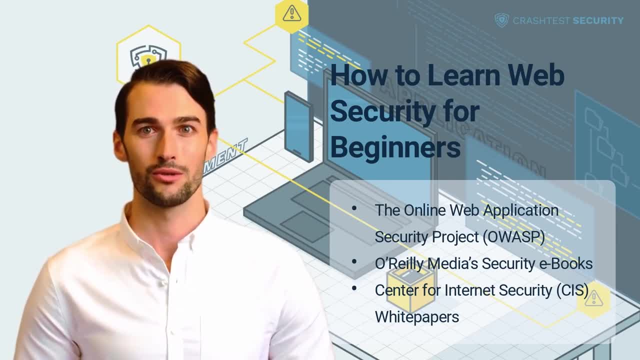 Software Assurance Maturity Model. SAMM, a recommended software model that helps administer, analyze and improve a secure development cycle. ZAttack Proxy, An open-source security tool that provides a wide range of options for application security automation. The platform also offers a marketplace that includes essential add-ons for functionalities. 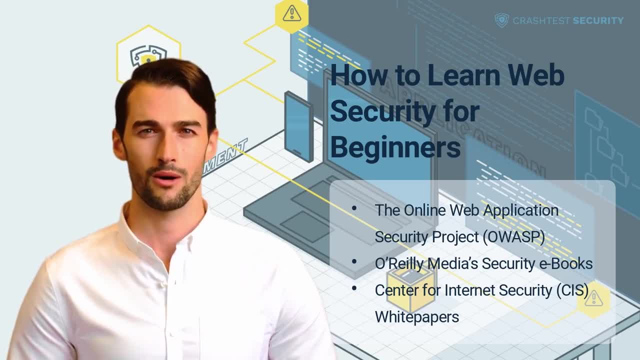 such as antivirus software, enforcement of strong passwords and support for IDEs. 2. O'Reilly Media Security E-Books. In addition, O'Reilly's Internet Archive includes several e-books on cybersecurity that consider modern security paradigms such as the Darknet, Data Lakes and DevSecOps. 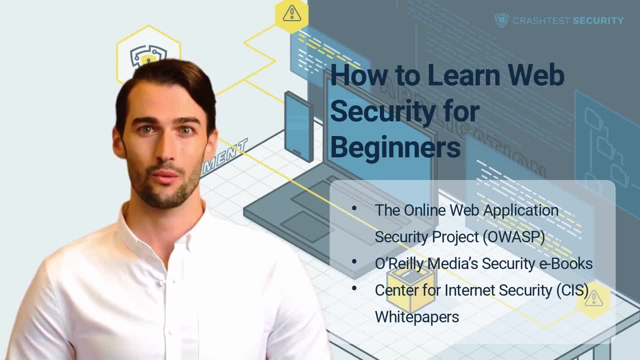 To access these books. you can sign up for a free trial to access a wide range of resources to gain information on the changing threat landscape, attack patterns and mitigation strategies. 3. Center for Internet Security- CIS White Papers. The Center for Internet Security includes a collection of up-to-date white papers. 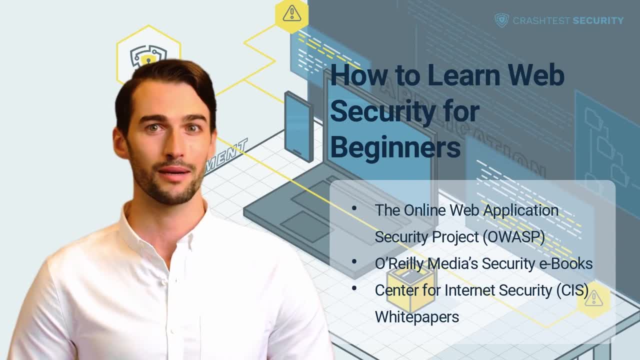 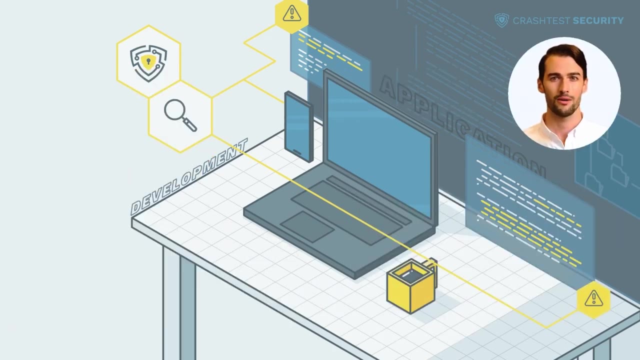 that help identify, promote and sustain cybersecurity best practices. This website also features educational videos, webinars and other valuable tools to help anyone interested in keeping their organization's infrastructure secure. Try Crash Test Security today to discover how it integrates into your development stack. 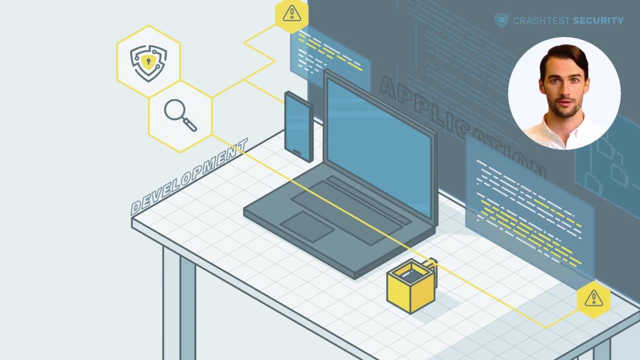 for efficient automated vulnerability scanning. The trial is free. Also, subscribe to the Crash Test Security channel and click the bell icon to be notified when a new video is uploaded. To get more information about the most significant web security threats, their prevention and how to use the Crash Test Security suite. Thank you for watching and see you in our next video.